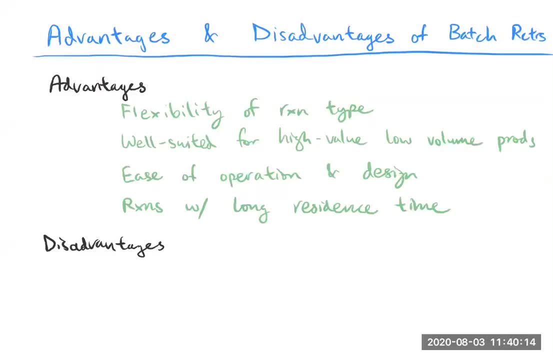 Okay, we've seen how to get at a batch reactor design equation and how to use it. briefly, And before we dive further into batch reactors, I think it now makes sense to go over all the different reactor types, But rather than just give you a bunch of, you know, derivations, 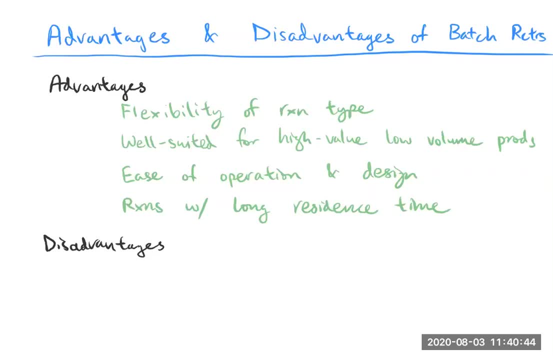 for different reactor types. I thought I'd at least start departing from batch reactors by talking about some advantages and disadvantages- And there are advantages and disadvantages for the other reactor types too. but for the sake of brevity, at least in this lecture, 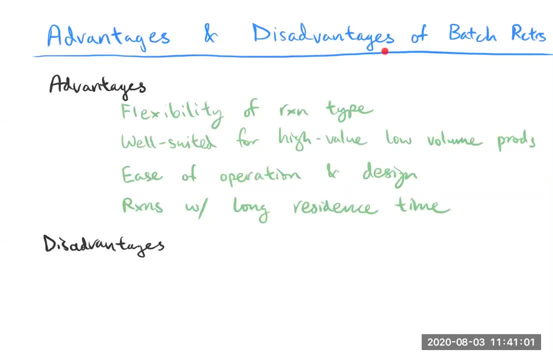 I won't go into all of those, But just to give you a sense of why you might not, well, why you might want to use a batch reactor first and then why you might not. We've talked about in O-1s, O-2s, O-3s, O-4s, O-5s. We've talked about O-1s, O-6s, O-7s, O-8s, O-9s, O-10s. 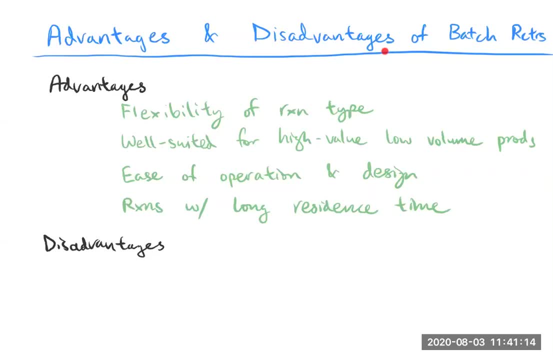 chem, organic chemistry or in your brewing cases, those are likely to be batch. So part of that is because it's really quick and easy, relatively speaking, to set up a batch reactor And they're flexible across a lot of different kinds of reaction types. So you know it takes a lot. 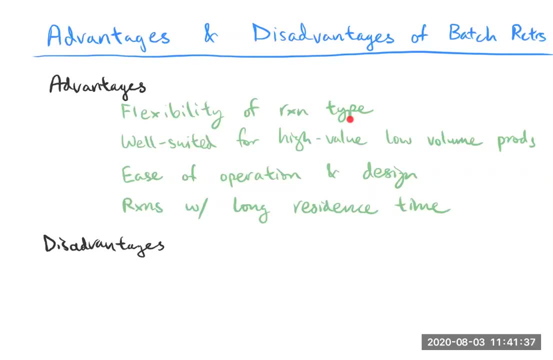 more effort and parts to get flows in and out And you know, there might be a variety of other reasons why you might just want to set something up in one vessel and let it incubate. A lot of times where you see this are for high-value, low-compound products, especially in the 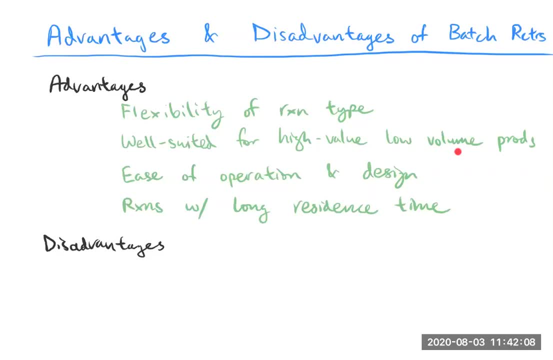 And so batch reactors may not scale as well, But they're smaller scales and when you need just small quantities of things, whether it's in a lab or, like I was saying, in a pharmaceutical manufacturing context, batch might be perfect for you. for that, I guess I already mentioned. 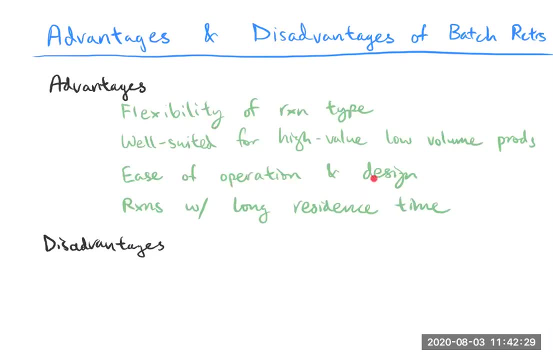 in regards to flexibility, some things about operation and design, how easy it is to set up. So I'm kind of mixing a few of these advantages um, including, for example, reactions with a long residence time. well, so um fermentation, the process where you have um cells um you know, ferment or make products um 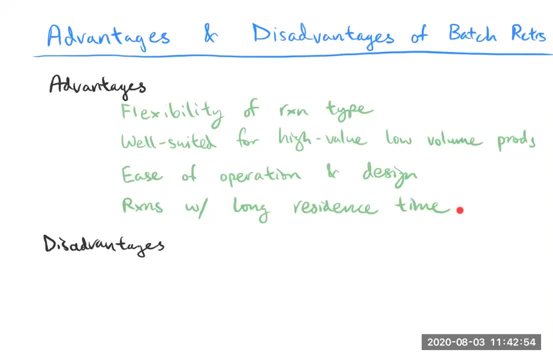 sitting in in in reactor vessels for a long period of time. um, that's actually how many of these high value, low volume pharmaceutical products are made. but just in general, if you need something uh to to be uh, incubating is a term that i'm using again here, um, for for a long 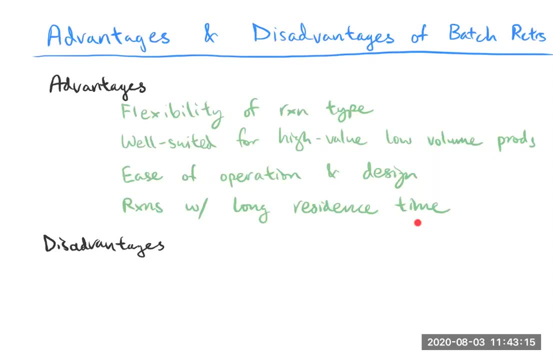 for for a long period of time. you don't want it to be pushed out of the reactor volume because of flow, um, and so those are some advantages, um, and and. so now, if we um think about some some disadvantages here, um, uh, one of the the the disadvantages that we might see is um, um, because it's not continuous. 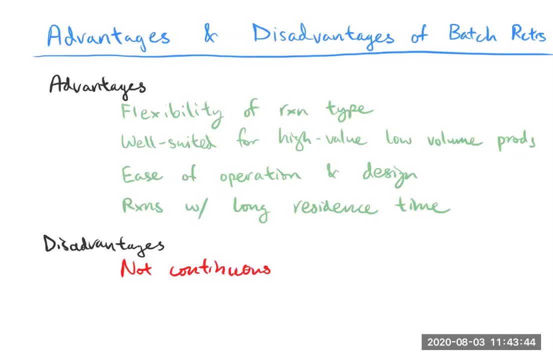 um, there has to be some element of downtime between batches. downtime between batches, um okay. so imagine that, um the the brewing case, um, where you're brewing, you finish making your batch of homebrew and then what do you have to do? you have to clean it out. 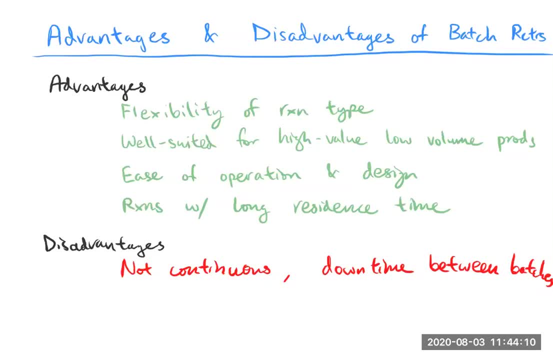 you have to sterilize it and wait for that to dry and all of that. so that's some significant downtime. think about all the the time that might add um in industry. uh, so we'll also mention here cleaning um costly, labor, intensive um. you know, this isn't really the most efficient way. 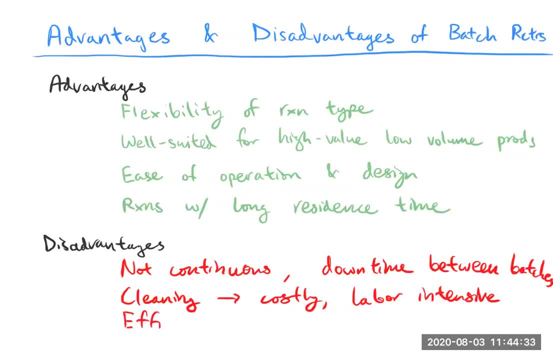 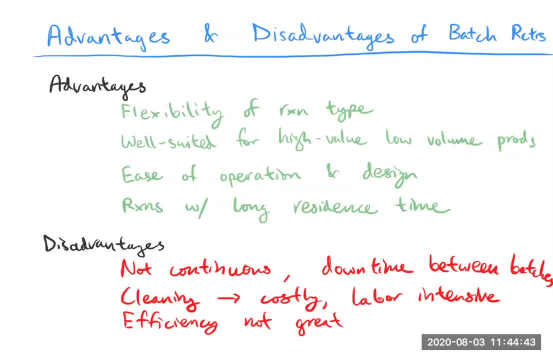 quantity of things and and use your time more effectively, maybe the volume more effectively, and we can talk about why that might be. then batch isn't really the way that you want to do that. and the other thing is at large scale, so large scale production, large scale production. 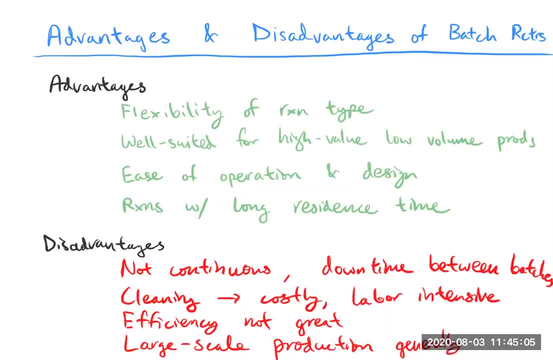 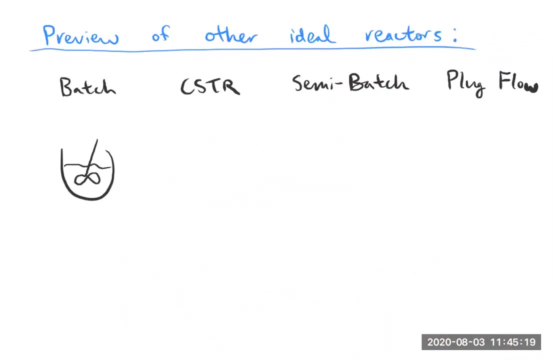 generally more difficult, more difficult. so those are. those are some disadvantages here of batch reactors. so let's go ahead and uh, look at um. uh, just a preview of um of different. so yeah, here here's your batch reactor, um diagram and uh and and term, and then you have your three other reactor types. 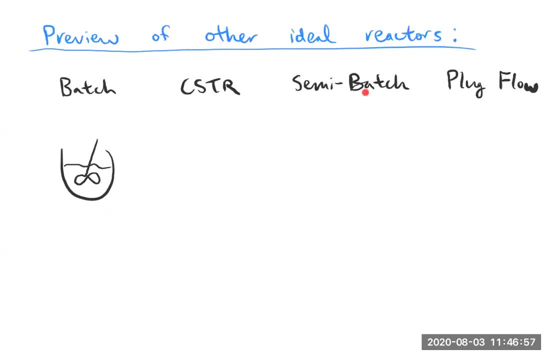 that are going to be of interest in this course. cstr's semi-batch plug flow, um, and so if we want to look first at what all these um uh diagrams might look like differently, um, we can start to draw out what a cstr looks like. so continuously stirred a tank reactor. so 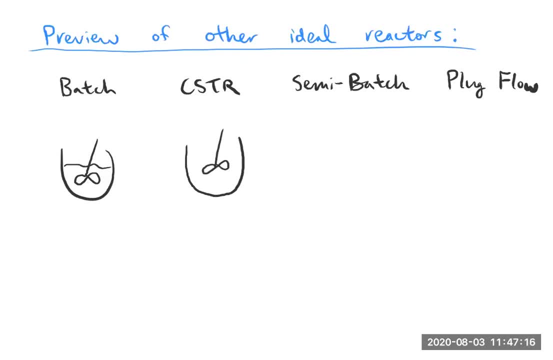 we're going to have a tank and we're going to have a stir um and now that the difference is that we're going to have um flow coming in and we're going to have flow coming out, what what um definitionally separates the semi-batch um from these? it's similar to a batch. 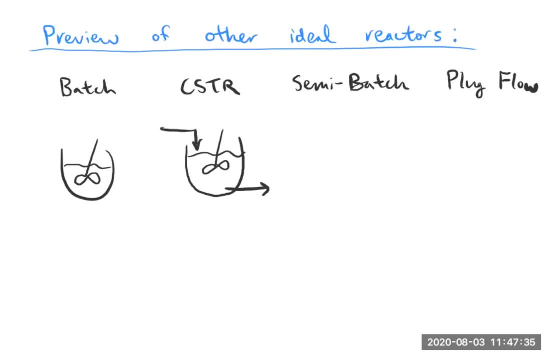 uh and a hybrid of a batch and cstr. so you have um once again, um, your, your vessel that's being stirred, and then you have um, just one um stream coming in, um and no uh, meaning that you don't have anything leaving the reactor. uh, no, flow out um, and then in the plug flow case. 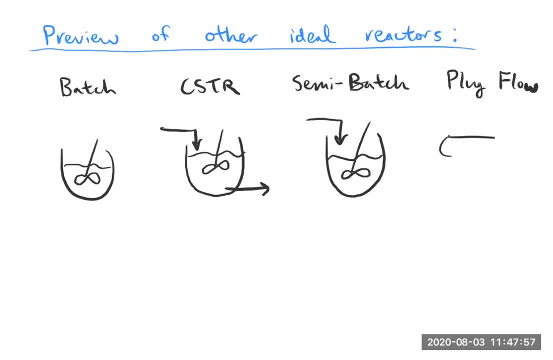 so i'll draw a tube, um, with an opening here, um, you've got, uh, so you've got a reactor happening essentially across the cylinder, um, and you've got flow in and out. and so now if we, if we try to say what, what's different in all these cases? um, you know, you in. 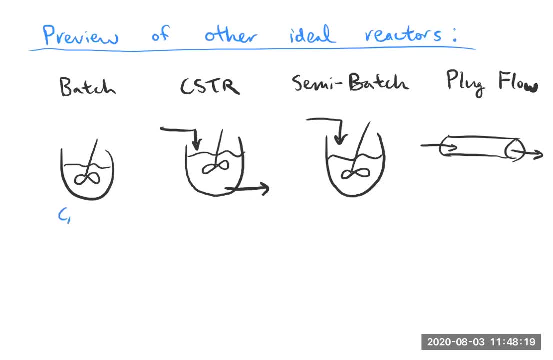 a batch, as we saw, you have concentration changing with time. um, you might also have um temperature, um, uh. so these um change with time. uh, your cstr, your continuously stirred tank reactor, one of the the definitional assumptions is that, um you operate it at steady state. uh, of course there. 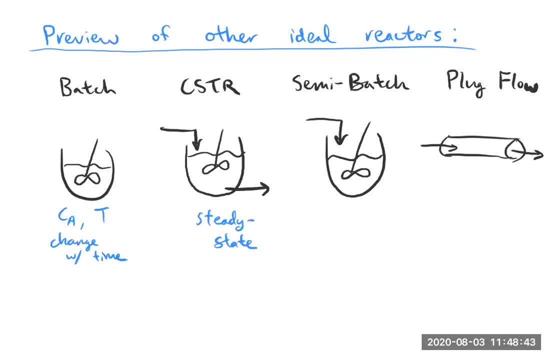 might be a startup phase, uh, in a shutdown phase, where it's not at steady state, but otherwise it is um. here you've got a semi-batch um situation where, okay, you don't, you don't have flow coming out, so it can't be at steady state, um, not steady state, um, in fact, it looks like your volume will. 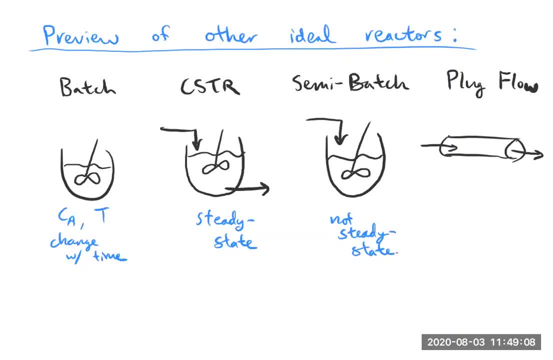 probably change um and then um. finally you've got plug flow, um happening at steady state, um, but um, as i highlighted in an earlier um video, you don't have, so not uniform um spatially, and so each of these different reactor types are things that you not only would commonly encounter. 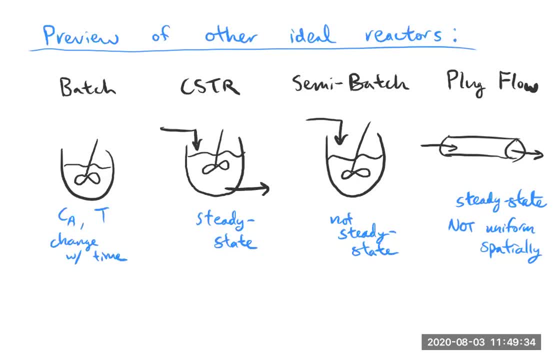 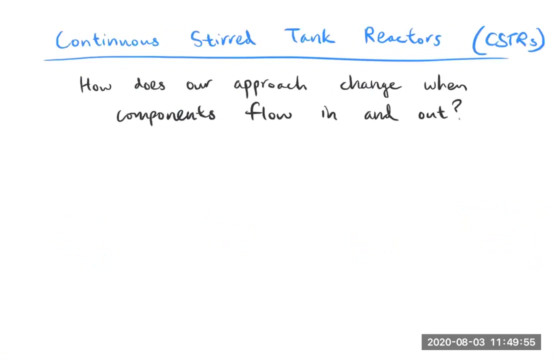 in in industrial settings, but they each uh throw a wrench into the, the generalized um balance, a little differently, forcing you to encounter a slightly different situation and then understand mathematically how to treat that. okay, so now, if we dive into cstrs, um, i'm gonna go ahead and and uh pose the question here. you know how does our approach? 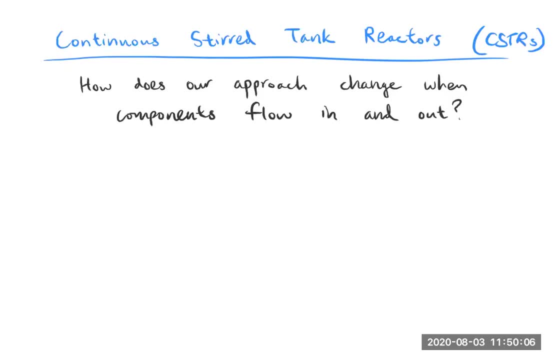 change when components flow in and out, and so i've already drawn a simplified representation of this kind of reactor, but i'll just draw it again here. um, you have flow going in and flow going out. you have a molar flow rate for your species. i mean, if you have a volume in and you have that out, if you're thinking about what's in your reactor. 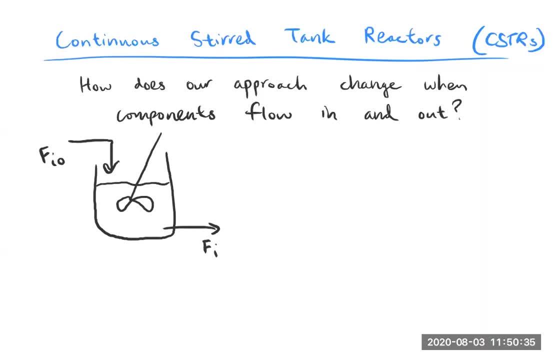 you've got, um, uh, you know, a given reactor volume, vr. maybe i'll just use a different color here to be able, so it's more visible. you've got, um, that net generation, of course, um, and you've got a given temperature that this reaction may be happening in. 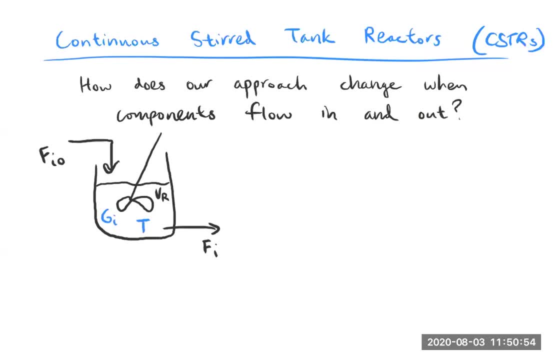 okay, um, let's talk about assumptions. so assume, assume one um, that everything is well mixed. um, so, continuously stirred, everything is well mixed within the reactor. all of those infinitesimal volumes, all dv's have the same ci and gi. okay, uh, what else can we assume here? 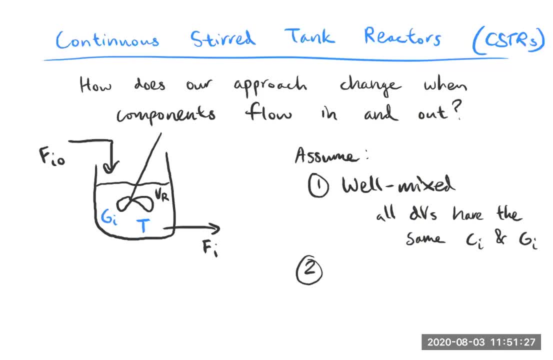 um, that um reactions only occur. reactions only occur in uh, vr, in the, in the volume of the reactor, within the reactor, um. so i mentioned that before. but you know, here it's kind of you might wonder, okay, well, if i, if i've said um had two fluids uh, 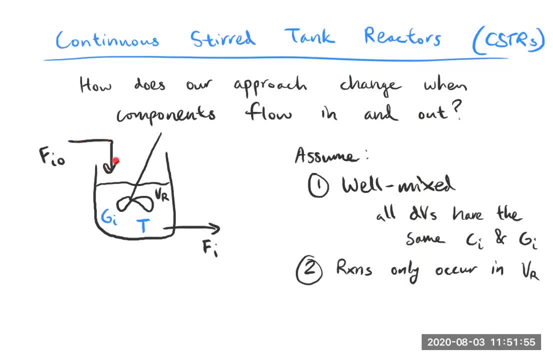 two separate streams of reactants come into a vessel and then they encounter one another and they start reacting and colliding, and they're both still present in the out stream. why wouldn't they keep reacting here? Well, you know, you just have to assume that they're not going to, and in reality, 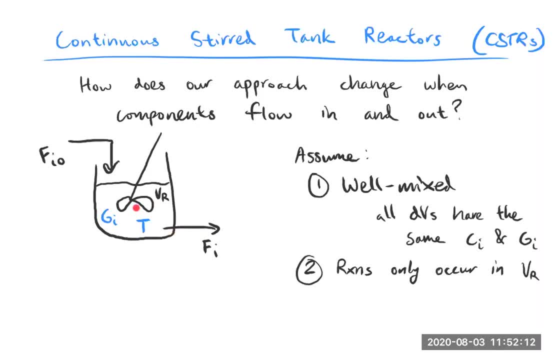 they might not, because maybe in your volume you have some kind of a catalyst that doesn't end up flowing out. maybe the temperature quickly drops in your out stream or you quickly encounter some other unit operation that effectively turns off this reaction. So there's also no reaction happening. if you've got a mixed stream coming in, it's only happening here. 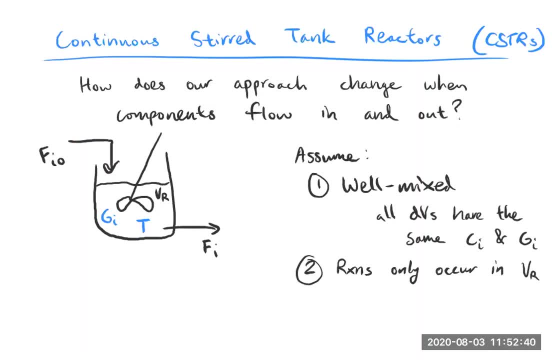 So what that means. so I guess I'll use the therefore symbol up there and I'll also say: here you have a step change in concentration in Ci, and I'll also say: and possibly T from feed to reactor. Okay, so just revisiting what I was saying before again. 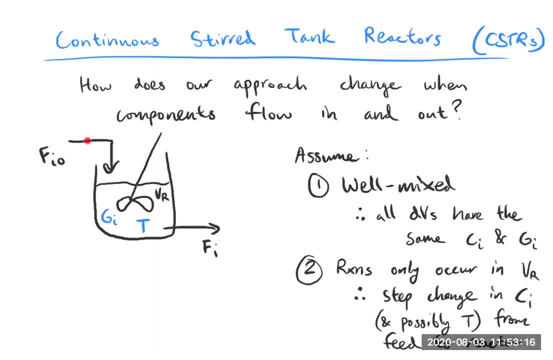 maybe you've got two components you know they're not reacting. They're coming in at maybe 300 degrees Celsius and your reactor is at 400 degrees Celsius. Well, okay, so there's a step change that happens. that you just say occurs right there, instantaneously. 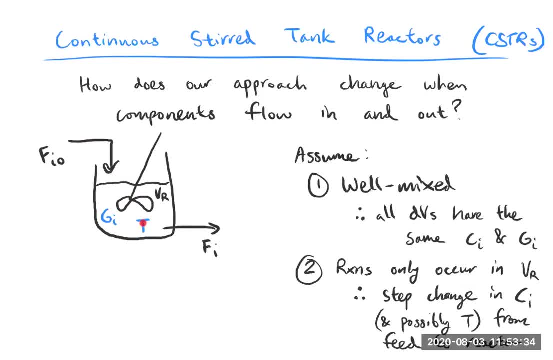 And you know, we're gonna also say, as a third assumption, I'll just move over here: steady state and those assumptions are are going to mean that our volumetric flow rate, little v out is equal to little v in, our vr is constant. okay, so, with these assumptions, we're ready to start using the design, the 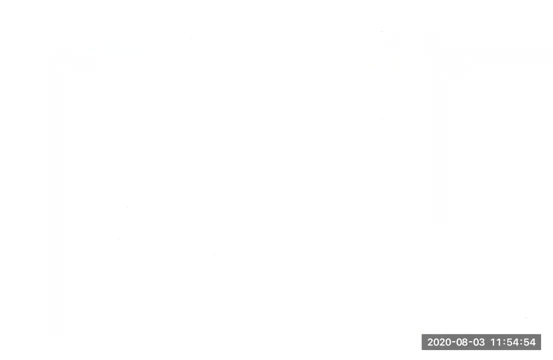 generalized balance, and so if we go back to what that looks like in minus out, plus generation, I'll just give that a net close assumption accumulation. sorry, we have an fi not coming in, we have an fi going out. we already said that our, our reactant is spatially uniform, so I'm just going to go ahead and write the net generation term. 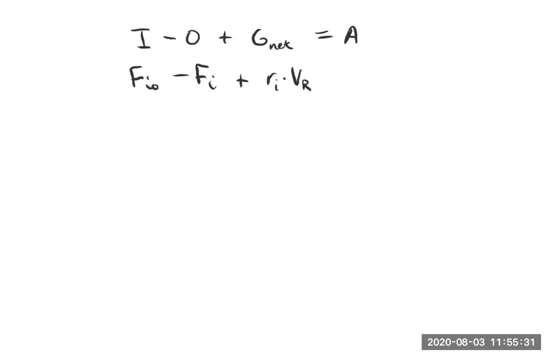 as the rate of formation of species. i times the whole reactor volume, sort of skipping a step from earlier, and our accumulation is still the number of moles changing per time. so dn, i, dp. now we said it's at steady state, so if that's true then we have 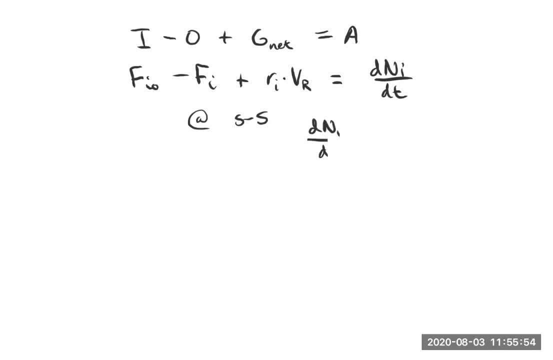 the. the dt equals zero. okay, so our derivative in this expression, uh, went away, and so we're left with now, instead of in a differential equation, just an algebraic equation. look at that. it's got three terms, though it's got more terms than we had before, and, and we know that um.